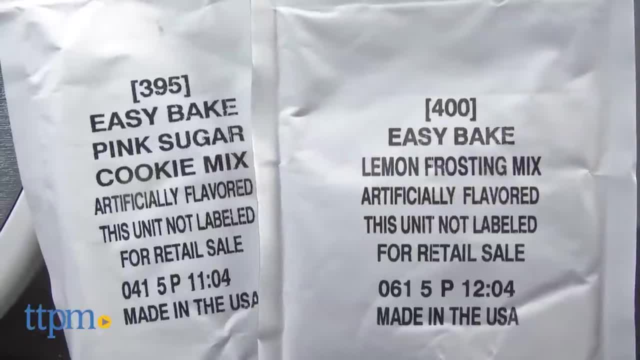 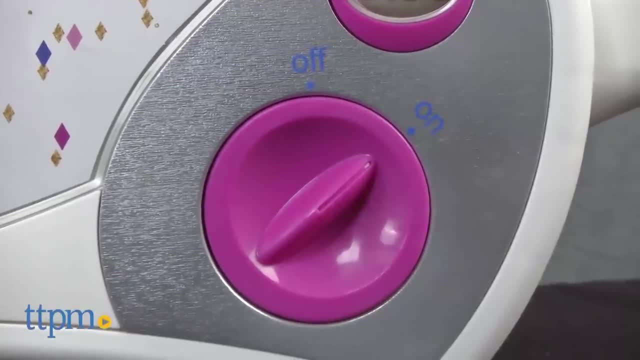 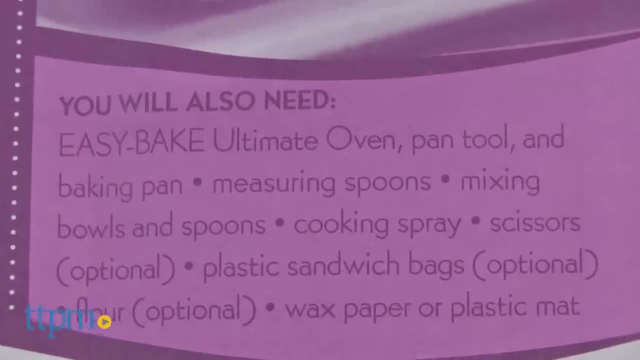 The set comes with three mixes to make three different treats: mini sparkle cakes, chocolate chip cookies and pink sugar cookies. It also comes with the electric oven, a special pan tool and a baking pan. To make the food. you'll also need some supplies from your own kitchen, including measuring spoons, mixing bowls and spoons, cooking spray, flour and wax paper. 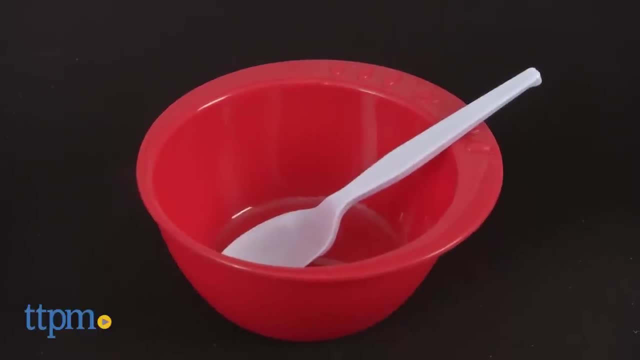 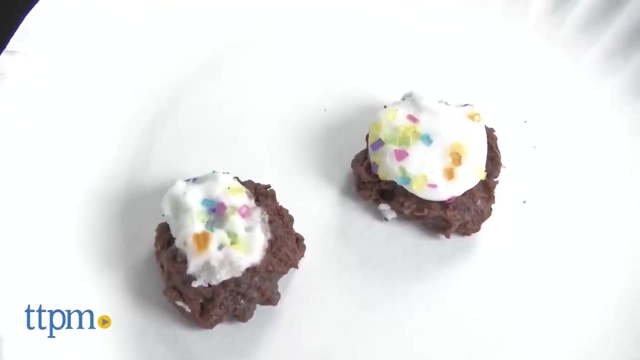 Though even using the most minimal tools like the plastic bowl and spoon we're going to use here, we were able to bake cookies. First, we made some mini sparkle cakes- The recipe makes 12, with six baked in the oven at a time. 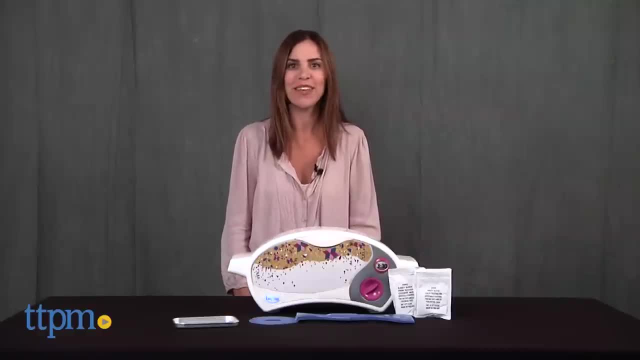 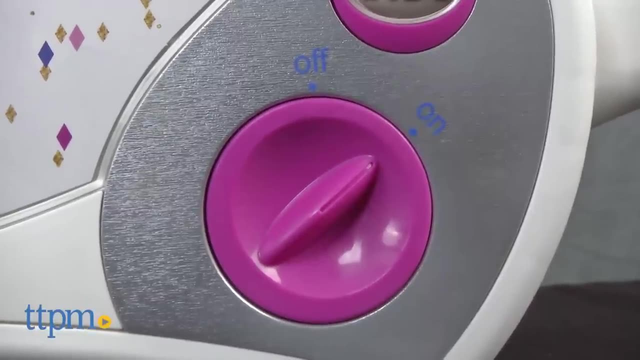 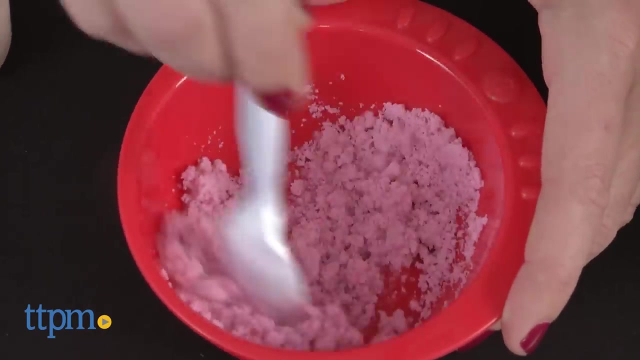 Now we're going to demo the pink sugar cookies using the pink sugar cookie mix and lemon frosting mix. We've already preheated our oven for 20 minutes, and now we'll follow the simple instructions and stir the pink sugar cookie mix with one teaspoon of water until dough forms. 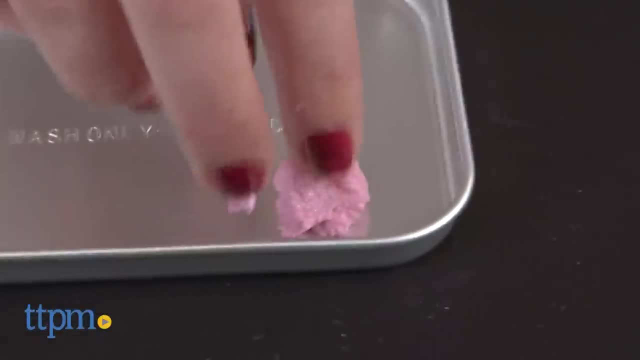 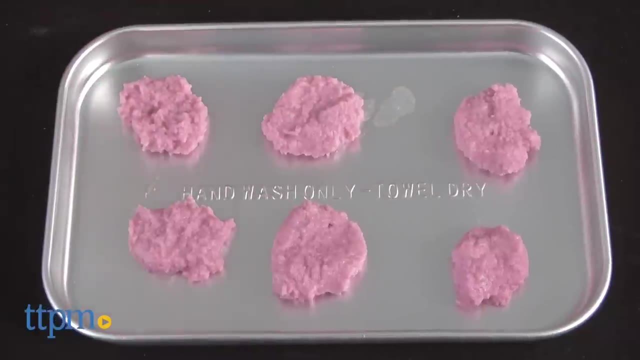 Then we'll shape the dough into 12 small balls and see how many we can fit on the baking pan, Flattening them so the cookies are not higher than the sides of the pan. It's that simple, and now it's time to bake. 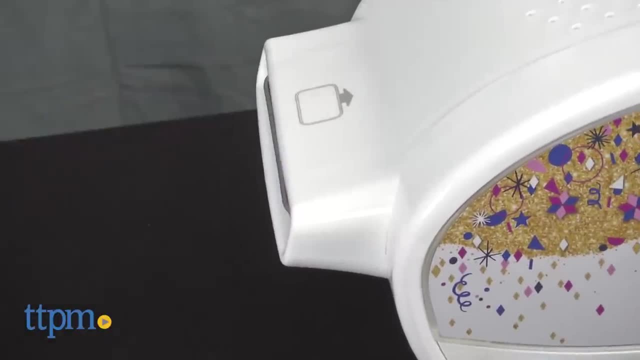 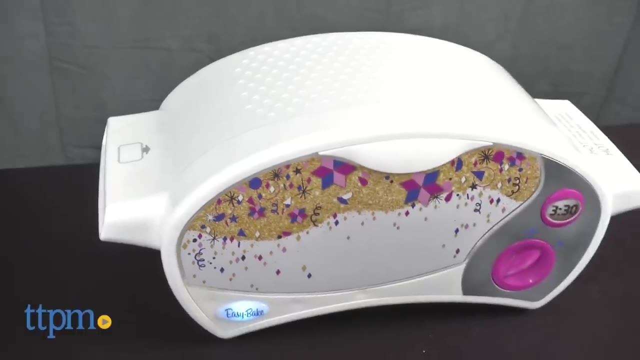 The recipe states baking time is nine minutes, though we found that we needed to bake the mini sparkle cakes longer than the recipe indicated, so let's see how these turn out. To bake them, you'll need to follow the baking basics on the back of the instruction sheet. 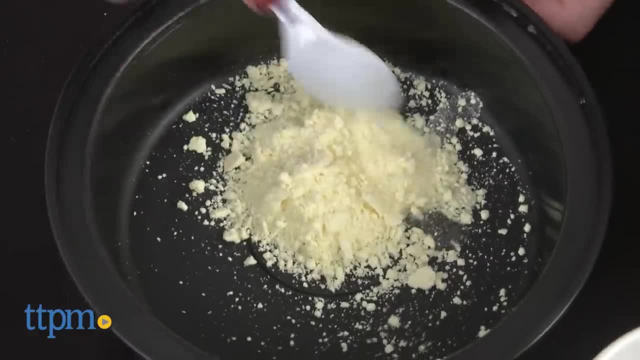 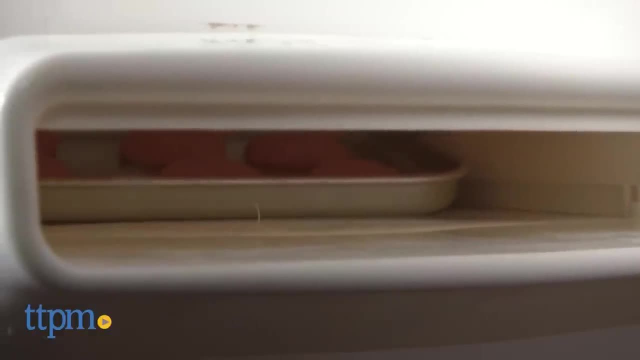 While they're baking, you can make the frosting by mixing the lemon frosting mix with half a teaspoon water until it's smooth. While the baking are up, carefully, move the cookies to the cooling chamber in the oven for five minutes, And when that's done, it's time to frost and eat. 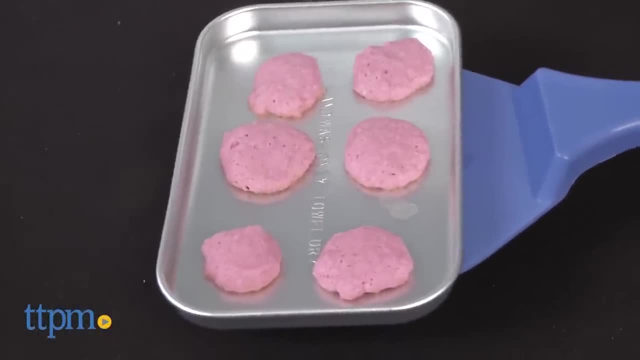 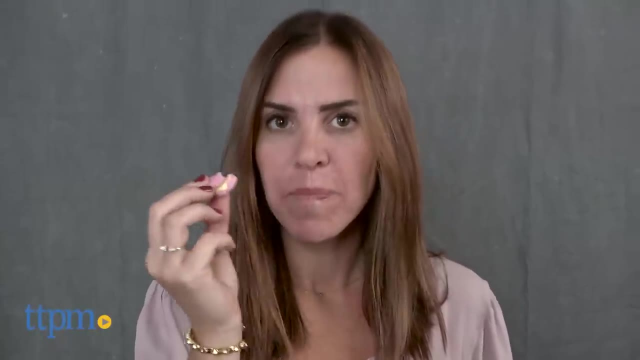 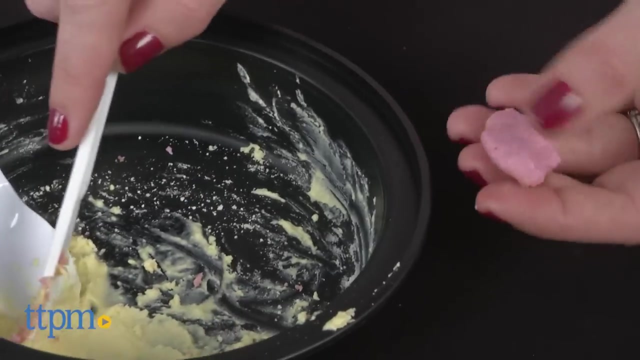 You can make little cookie sandwiches or just use the frosting as a dip. I'm going to try a cookie sandwich. Mmm, It tastes really good, Very sweet, but it's supposed to From sweet treats like these to savory staples like cheesy pizza. 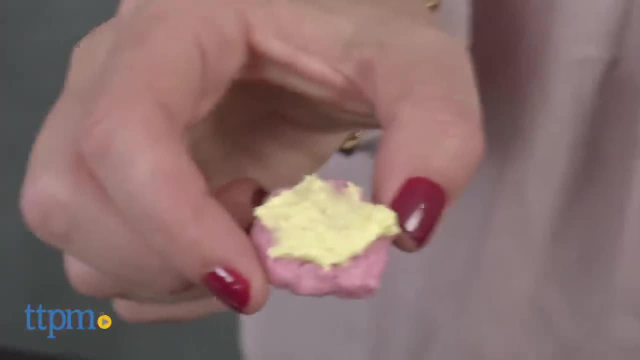 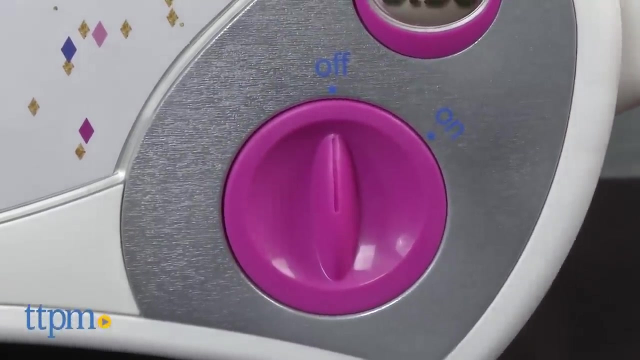 the oven is easy to use and helps encourage kids to bake. It's recommended for ages 8 and up, though adult supervision is required, since it is an actual electric oven For where to buy and current prices. find us at TTPM and subscribe to our YouTube channel for more reviews every day.